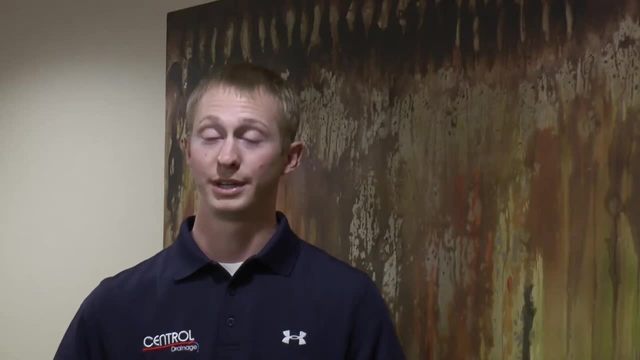 The next step would be to get a healthy plant growing. which tile allows That? because you now create the optimal soil environment Each spring. you have the oxygen there, you have the water there, because the tile lines move the water table and the excess water. 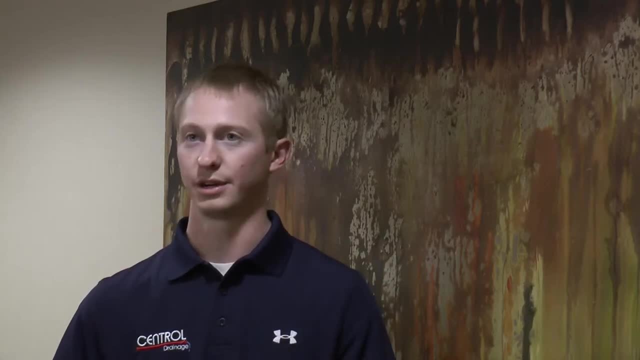 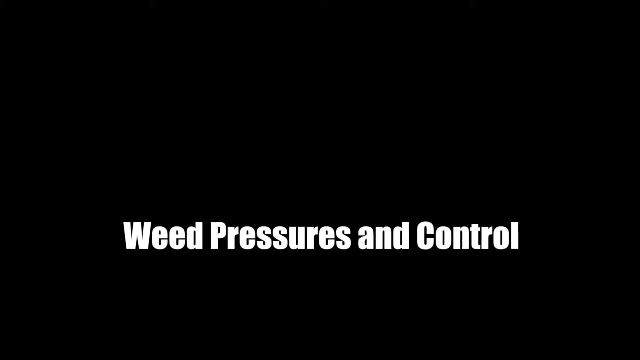 out. So after the healthy plant starts growing, now you look at, start leaving the residue. Residue in turn then forms soil, organic matter and that over time helps you build better soil structure. Then you can start leaching that excess water in the salt through the profile. So of course one of 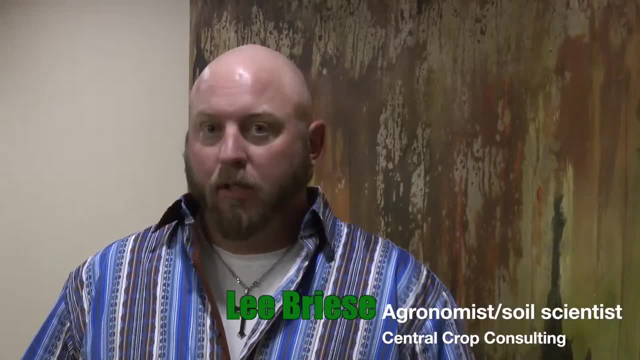 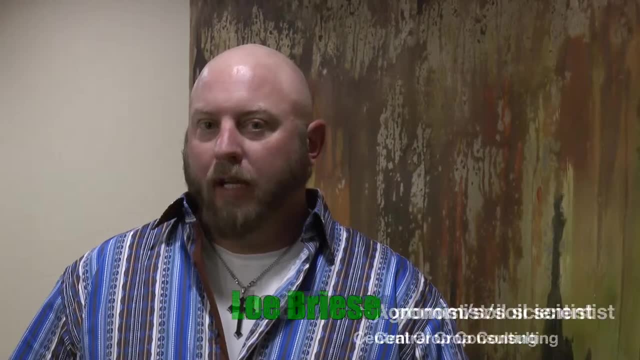 the major tools that we have for us. without tillage is a herbicide, but it's only one of the tools that we have available to us. I'm encouraging the producers to look at all their entire system and to use those tools as an effective management things. Things like crop canopy, row spacing. 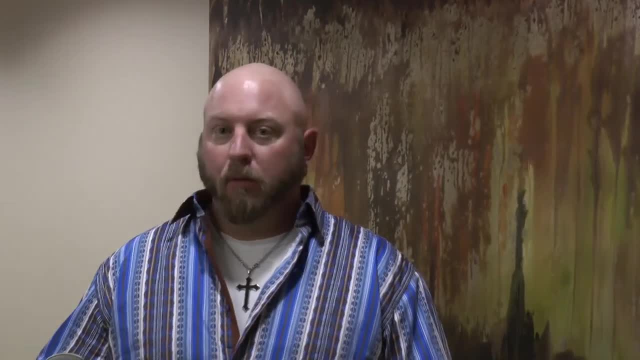 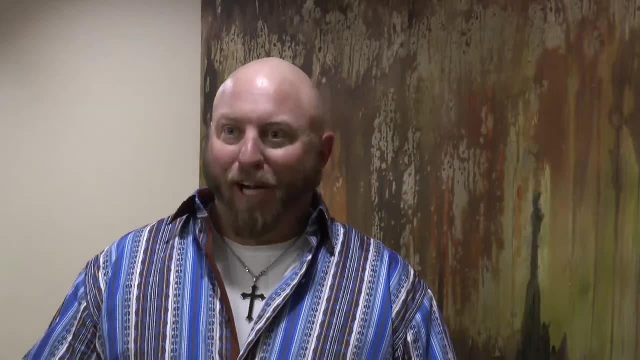 cover crops. those are all parts of it. Even residue management can be a weed management tool if you use it as a mulch and use it effectively. But you have to have it as a weed control idea in your mind when you're running the combine. You can't think about it later. 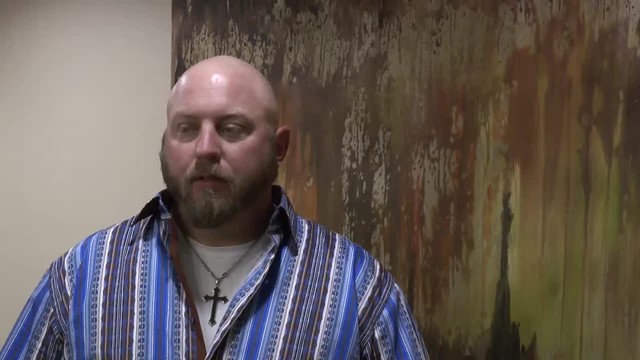 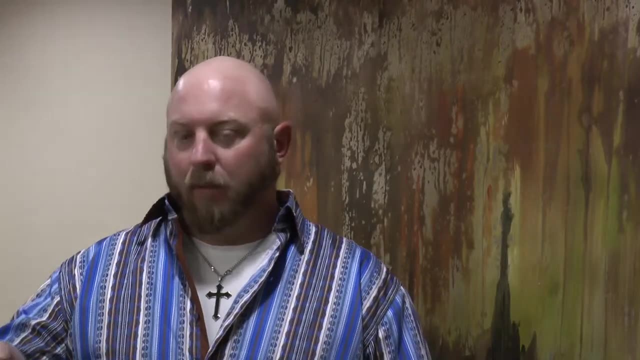 One of the things with strip-till is that you're going to have two different sets of places. You're going to have some high residue areas and you're going to have some low residue areas. So you're going to have a difference in temperature, you're going to have a difference in moisture, you're going to have a difference in emergence. I think it's really beneficial for farmers to be aware of those differences and then to plan with them accordingly. The vertical till system can actually cause a really quick flush of weeds at a certain point in time, If it's done at the right. 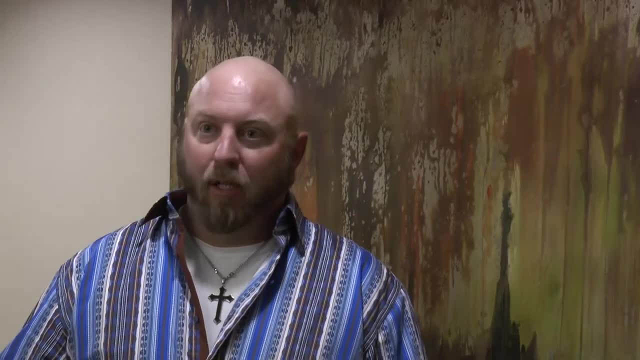 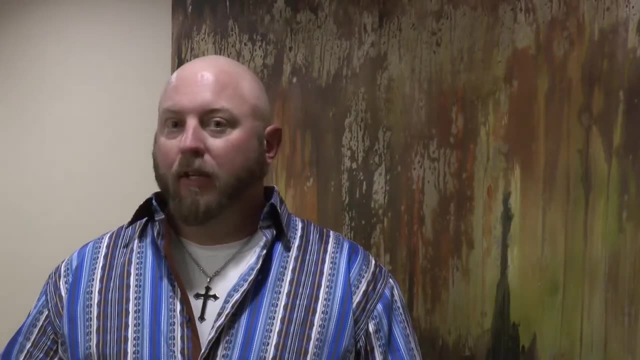 time. so you have to be really ready to react very quickly and understand that the vertical tillage pass can cause a quick germination of weeds. If you're looking at using a pre-emerge or something else, you need to be on the stick and ready to manage that Weeds and no-till. I think it really. 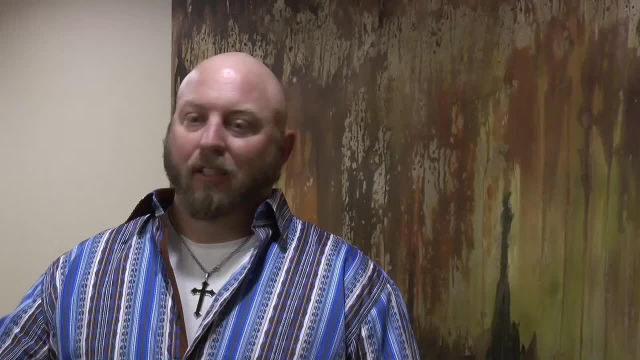 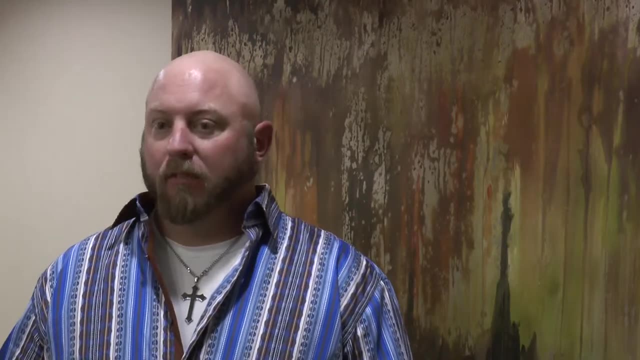 is important for that multi-prong tool. You really have to look at a number of different dynamic things and understand the nature of your no-till soils- And each no-till is going to be different, each field is going to be different- But identifying the specific weeds and then you can. 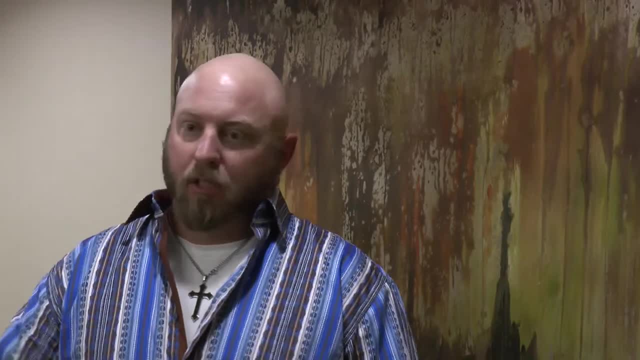 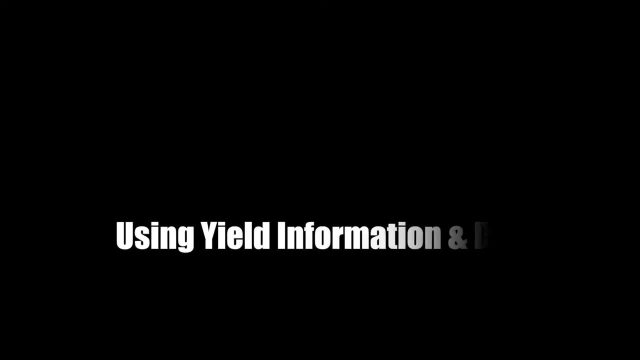 match your tools to the trade, whether it would be using the residue, whether it's going to be using a cover crop, whether it's going to be using a different crop that's going to be more competitive for a period of time. Those are all parts, So all this information.